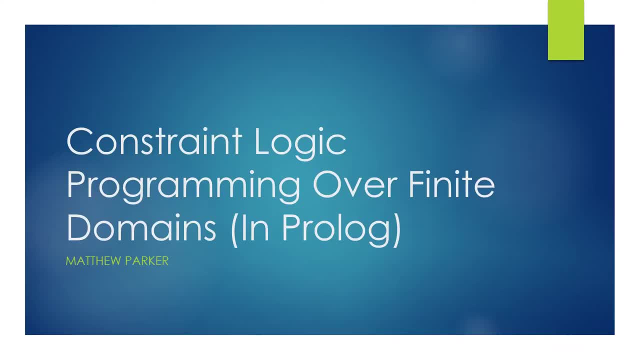 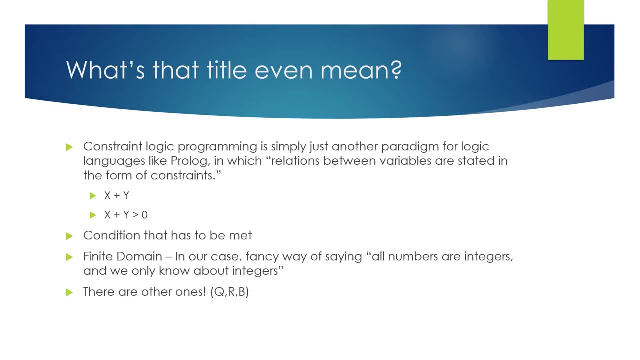 Hello, today I'm going over something called constraint logic programming over finite domains and prologue, and some of you might be like: what's that even really mean? because that's just a big jumble of words really. So constraint logic programming is basically saying it's a paradigm. 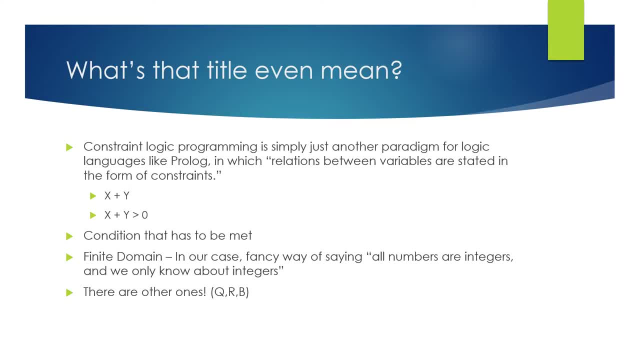 where you add constraints to your variables. So in the first example here you have x plus y. it's without constraints, so it really doesn't mean anything in this paradigm, whereas the second example there shows x plus y is greater than zero, where the constraint is that their sum is greater. 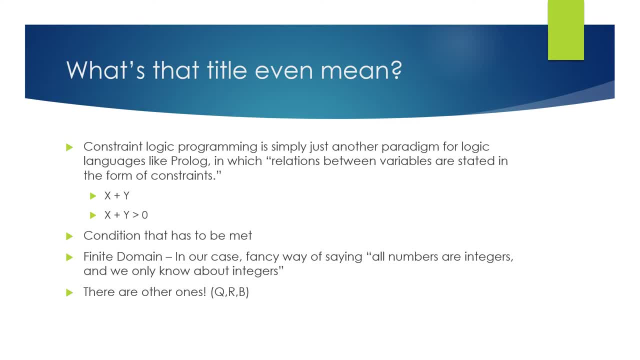 than zero, and the idea is: all constraints must be met when you're programming this paradigm, and the finite domain part is the really odd sounding thing. Really, it's just a fancy way of saying that everything we're dealing with's integers and that's all we know about when we're 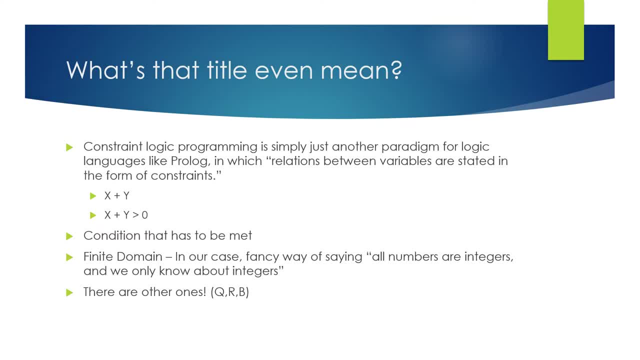 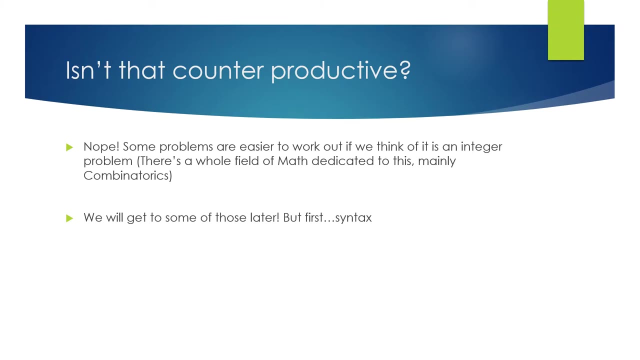 using our um, our constraints, and uh, there's more than finite domains. you can also do your rational numbers, your real numbers, and there's booleans, but we're not really talking about this today. So some of you might say, why would you only want to work with integers? isn't that kind of 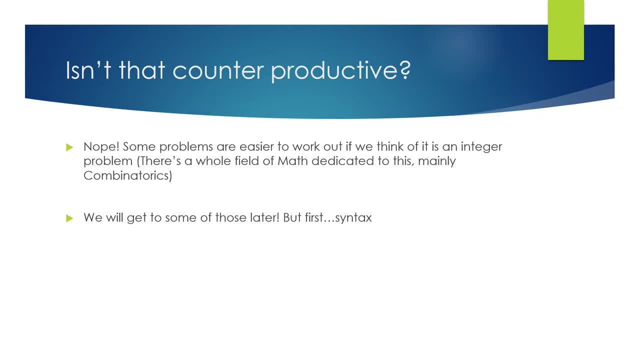 counterproductive since, like you can do a lot more with real numbers and really no like this, there are a lot of integer specific problems that this actually helps address and there's like the whole field of combinatorics and math is actually dedicated to solving problems like 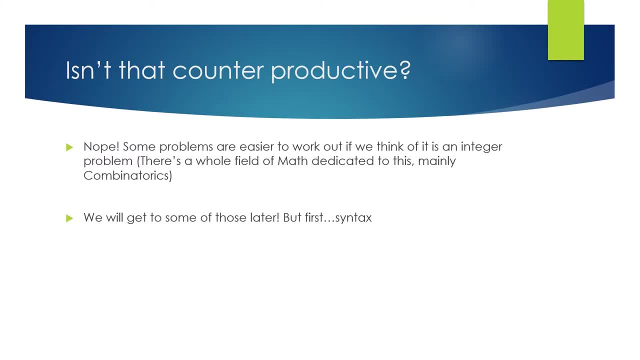 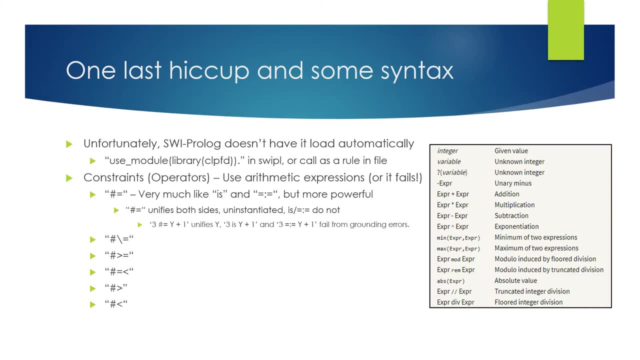 this. but before we get into how to solve these problems, I want to go over some syntax. So prolog won't swivel anyway. it's kind of dumb in that it doesn't load this library automatically. other versions of prolog will, I think um GNU prolog might, but yeah, you use this. 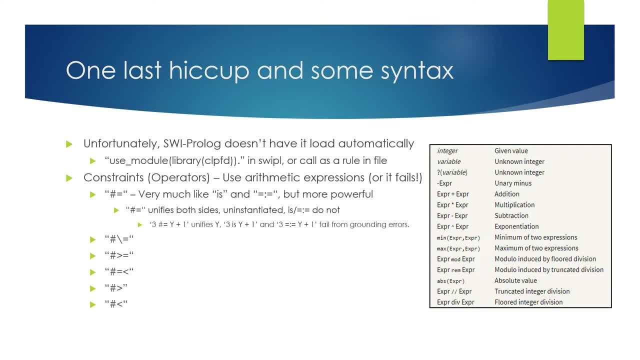 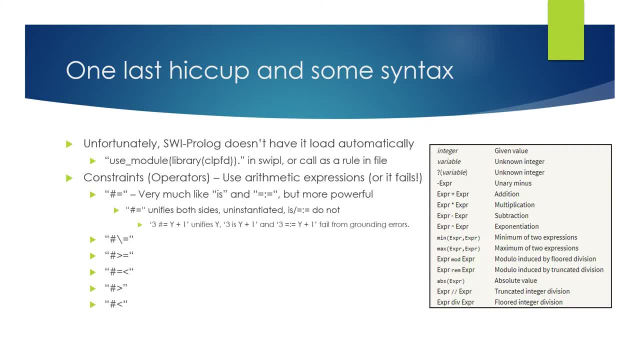 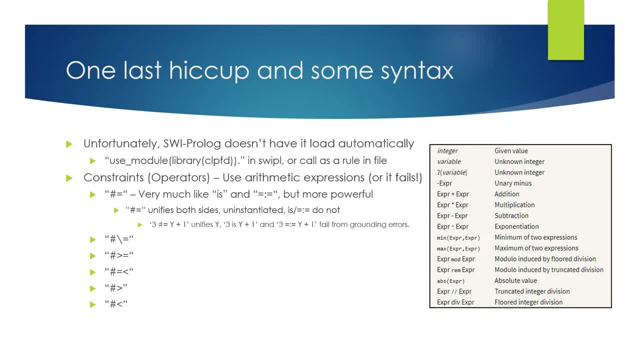 And doließ这全部重覚我们这个温馨 либо和可以做这样的 things that are called constraints, but they look a lot like operators that you've seen before. super noticed these speakers getting점 the technology stuff. they change over the. 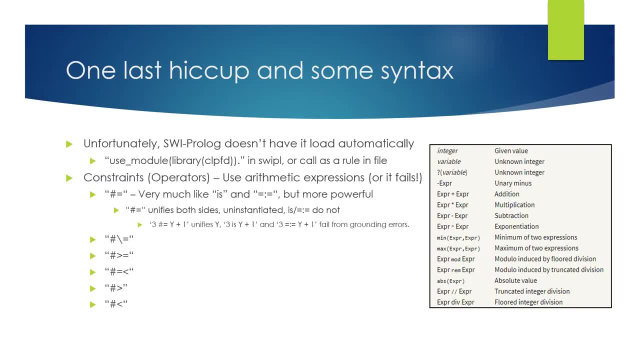 something like using a Scott as met at expressions which are everything you think. Note the technicalacht Beer people at mem🤘. right, any one of these things could be seen as an arithmetic expression. If you put in something that isn't one, it automatically fails and yells at you. So the first one looks a lot like. 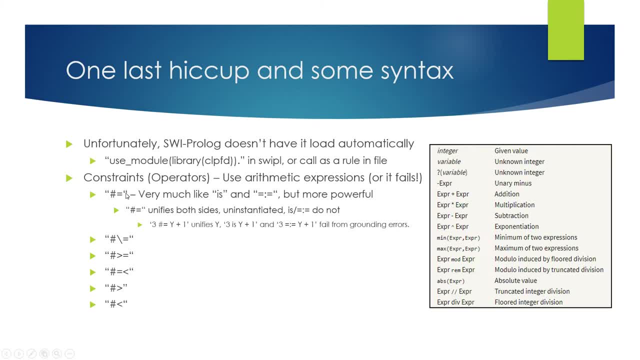 unification and it's kind of similar but not really. It acts more like the is and the equivalence predicates, but if you use both of those predicates they only unify one side. So if you try to do three is y plus one or three is equivalent to y plus one, it fails and yells at you saying that: 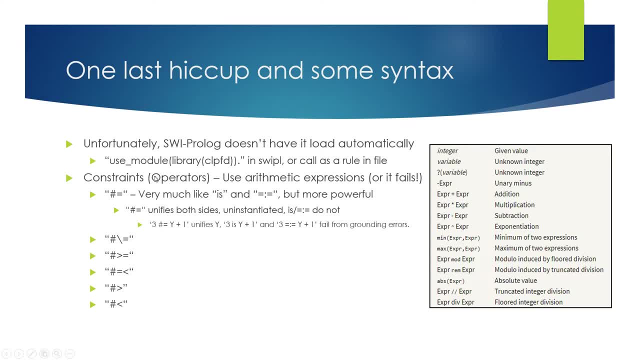 there's not enough things that are instantiated. With this constraint, however, it'll be fine with saying y is two, for example. And then we have other things, such as you know, not equals, greater than equal to, equal to or less than greater than or less than The standard things you'd expect to do. 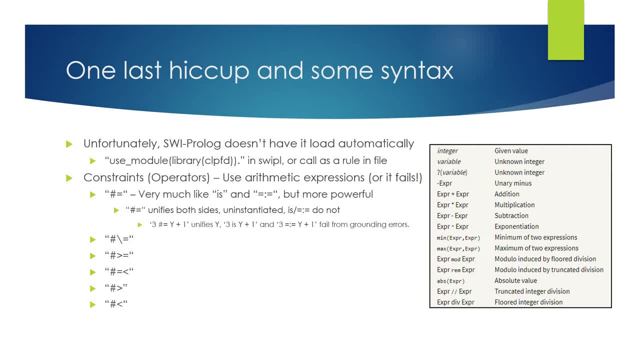 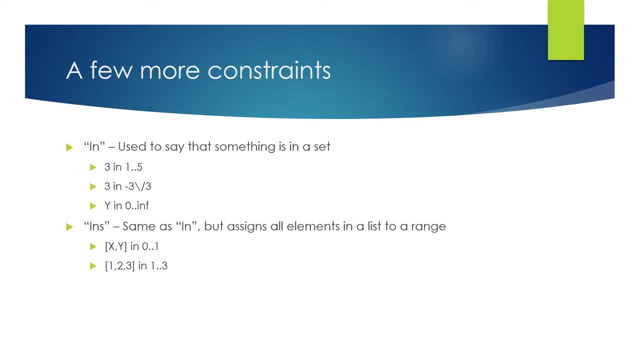 like the standard- excuse me- constraints you'd expect with arithmetic. So there's a few more constraints that we can do, which are more or less set constraints. So the first one is in and you can. there's a few different uses. You can do three in the range from one to five, which is an inclusive range. so it 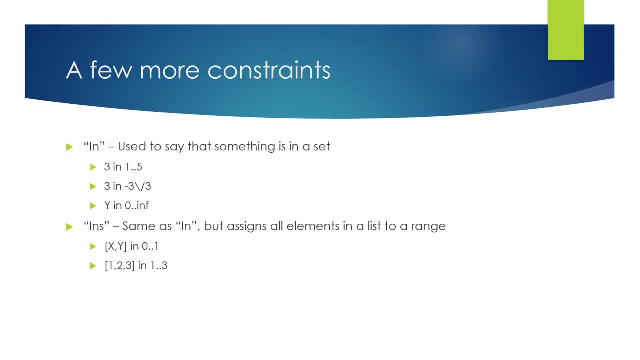 says is three in the range one, two, three, four or five. So then it's true, Three is in the disjoint between negative three and three. So if anyone's taking a class that has to deal with sets in mathematics before, this can be seen as the union. 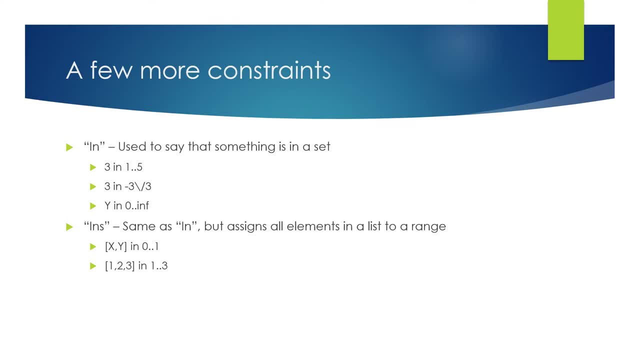 between sets, where there's a set negative or a set containing just negative three and the set containing three. So since three is one of those elements, it will be fine with it, And then we can say: y is in the range from zero to infinity, But without other constraints. that's all we know. 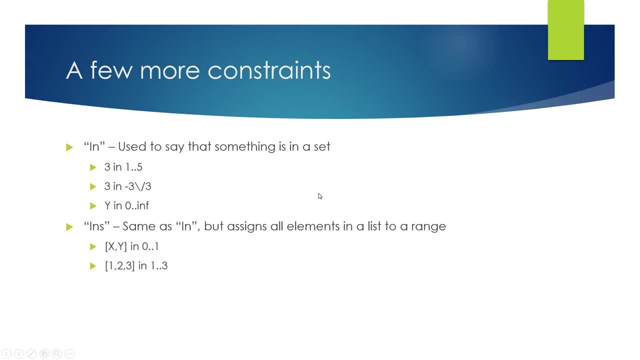 about y. Then there's another one called ins, which is basically the same as in, but it will put every element in a list to that range. So on this first example it will end up doing: x is actually mistyped, that should be ins, and ins It will say x is in zero to. 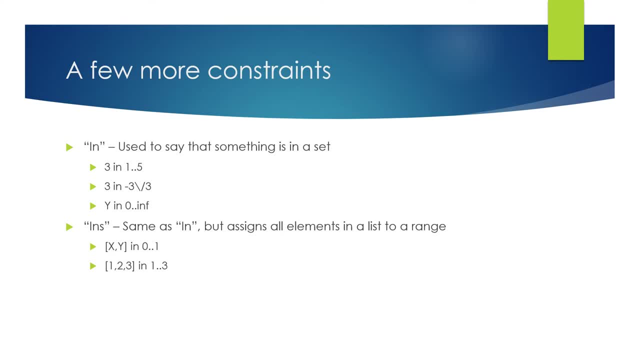 one and y is in zero to one and put the constraints on each of the elements. This thing is basically saying: is it true that the elements one, two and three are all in the range of one to three? You do want to know that they are wyned. So if you do that, it's going to become very 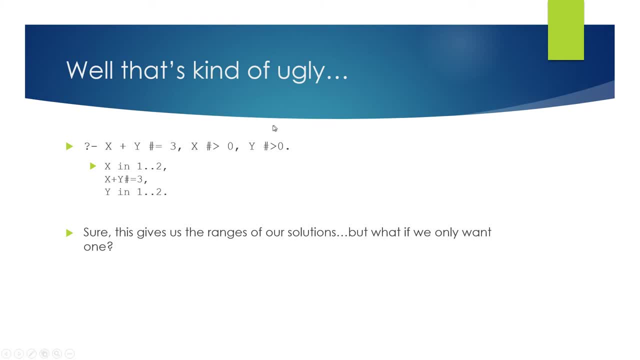 try super hard language by that one. so these two conditions are going to be kind of hard for you And in fact if you kind of just type with constraints in queries like this, saying you know x plus y is three, You want an x. 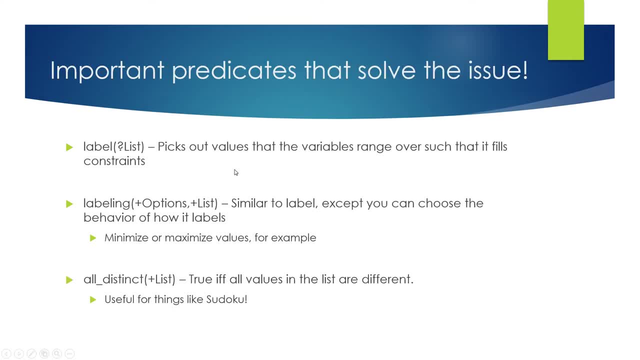 greater than zero and y greater than zero. It kind of ends up getting ugly And it just gives you the ranges. So there's a solution- this I'm going to get to that next slide, but this really isn't useful. So 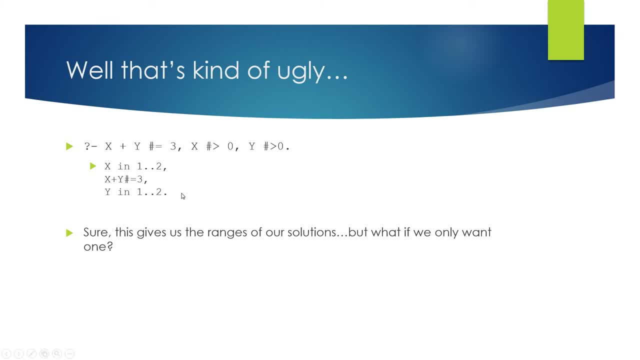 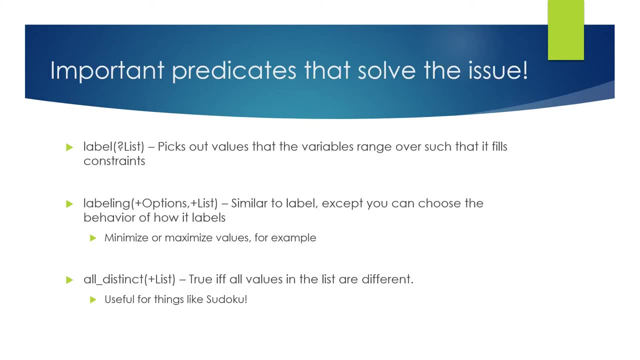 is. you know, x is 1,, y is 2.. Those add together to make 3.. And then another one is: y is 1,, x is 2. And, as we'll see in a moment, label will actually show all of. 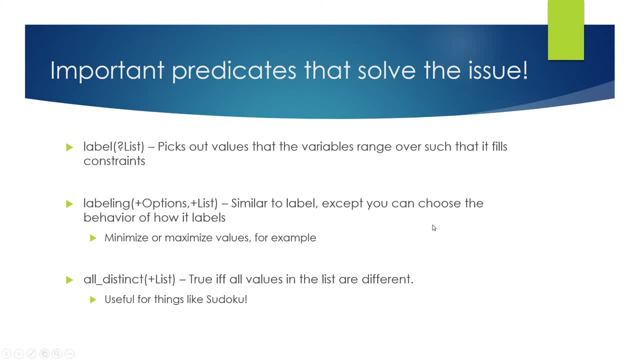 the solutions. There's another predicate called labeling, which allows you to add more constraints to how you want your output to act. So you can make it so one variable is maximized first or minimized first, and a few other things. I don't want to get into too much detail there. And then there's one more, really. 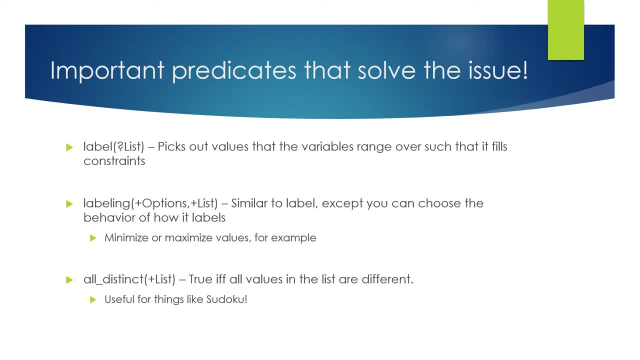 important predicate called all distinct, which will tell you if all the elements in a list are different, And that's useful for problems like if you want to solve Sudoku, for example, There's nothing in a row, a column or in one of their. 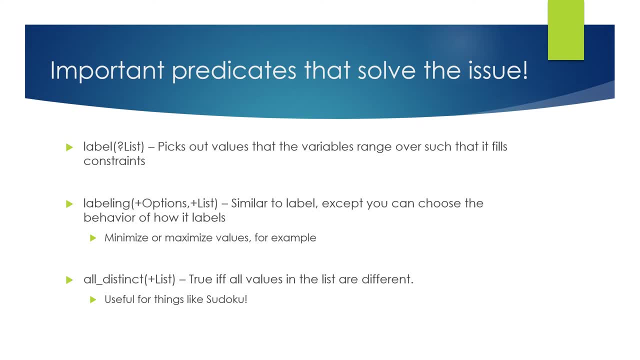 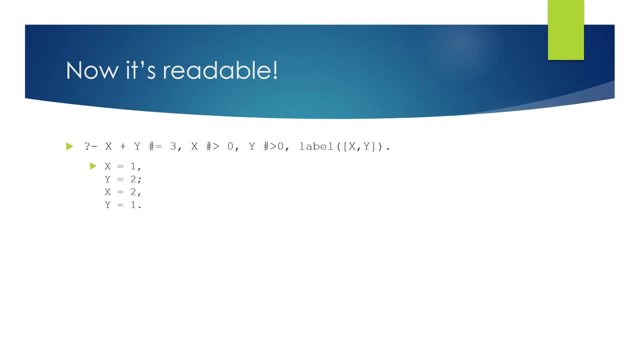 3x3 grids that can't like. all the elements have to be distinct. So if we add this label thing, which is something that we're going to call label the variables x and y before you end, it gives you the two solutions I was 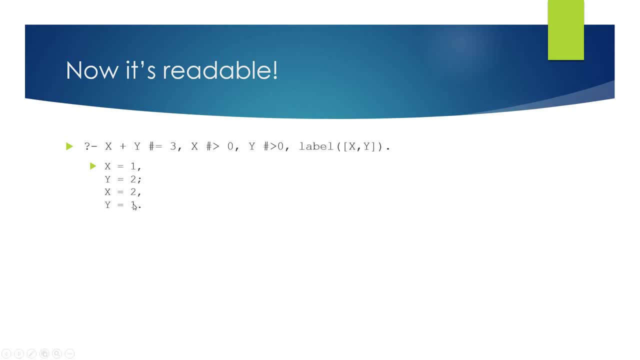 saying x is 1, y is 2, or x is 2, y is 1.. So here's a kind of interesting problem you wouldn't actually really think about solving. So you have this map right here and you want to color each one of these cells. 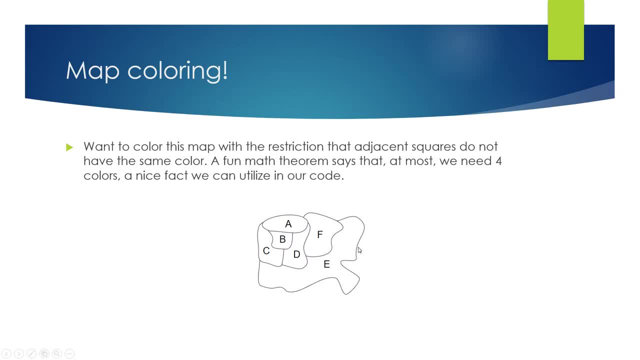 that's labeled with the letter Colors, such that if A is touching any of these things, none of these things are the same color as A. And when we're doing this, there's a nice thing called the four color theorem. I don't. 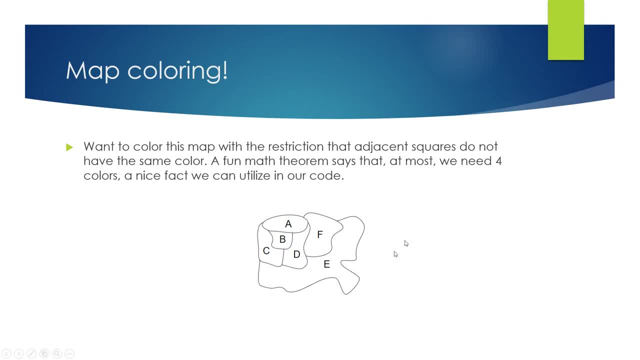 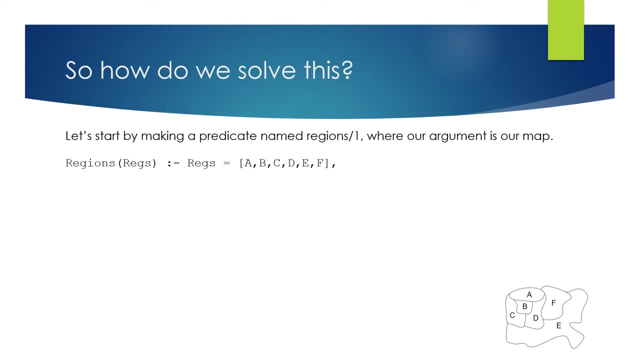 want to get into that, but it says that at most we need four colors, And that's useful when we're actually coding this. So the first thing we want to do is make a predicate called regions, which is with a list that represents our map. So we 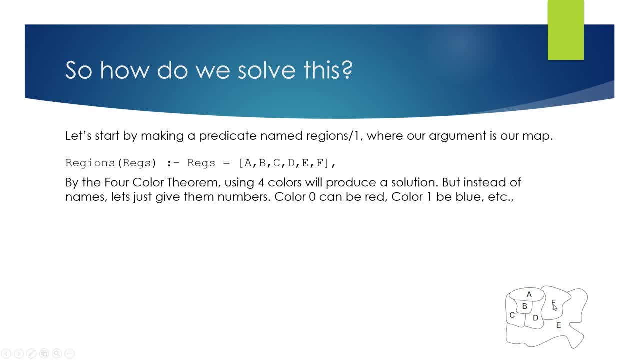 have the region A, B, C, D, E and F, And then we know that each color can be represented by a number. So let's say, you know, zero is red, ones blue or whatever. By that we know that each element has to be in: um sorry, each one of these. 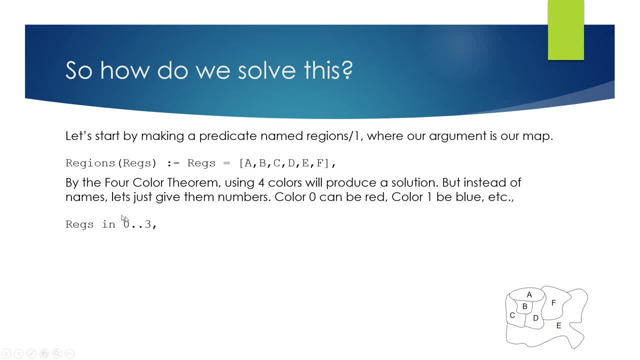 things has to be within zero to three- And I actually mistyped here. this should be ins- And they can't have the same color if they touch, so we actually have to put that constraint in it. so here are all the constraints we see. a is not the same color as 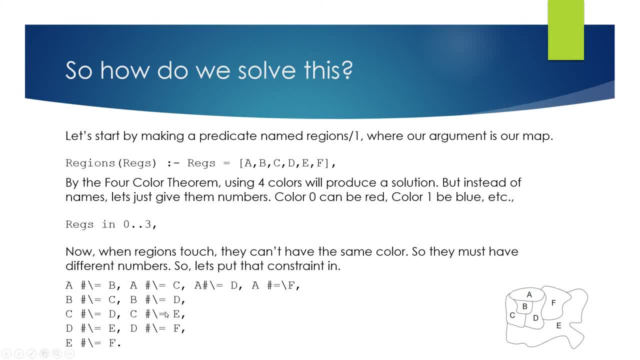 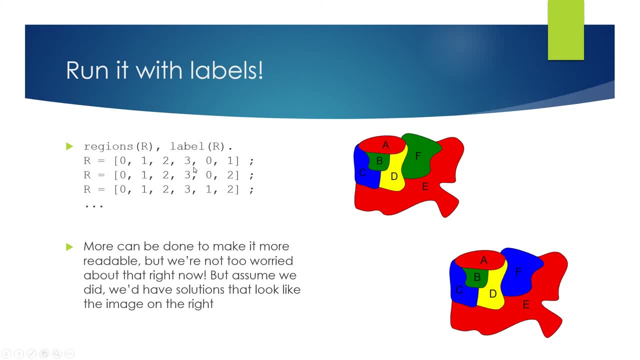 b. b is not the same color as c, etc. and if you run this normally you get a bunch of stuff that really doesn't make sense. so you end up having to run label with this and when you run it like this label give you a nice solution. so a has whatever color zero is, b has color one, c has color two d. 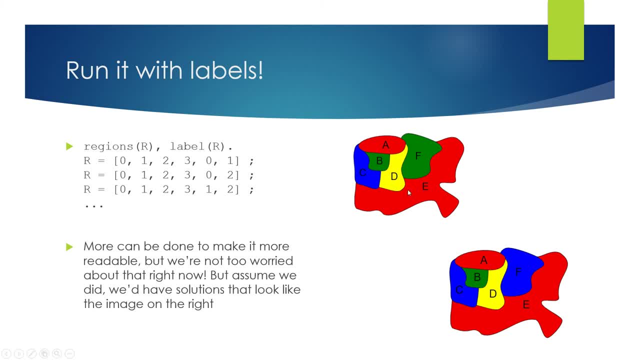 has color three, and then, um, he's got color what is it? zero, and this has color one. so this map actually shows this solution where eight- you know, zero's red, one's green, um, two is blue, three is yellow. and then here's another solution that i don't know which one that actually corresponds.